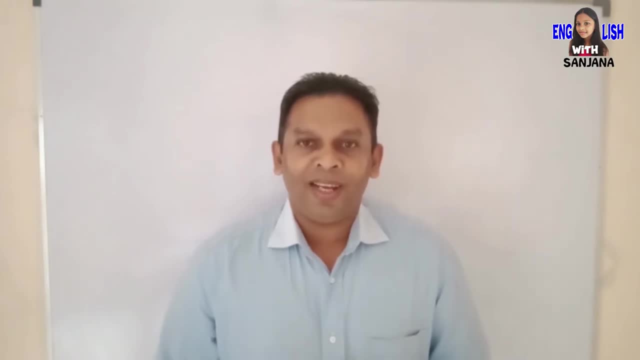 this video. First we will be looking at present population in the Asian region. Next you can have a general idea about the unequal population distribution in the Asian region and some physical factors that have impacted this unequal population distribution. Then we will move. 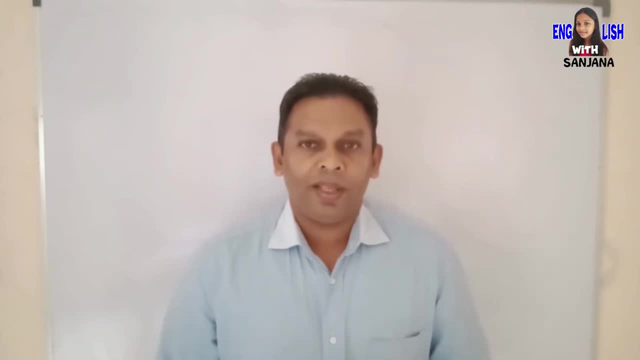 on to learn about some regions in Asia. Some regions in Asia are highly and densely populated, whereas some areas are sparsely populated. As the final content in this presentation, you will be reminded of 10 countries with a higher density of population and 10 countries with a lower density of population. I have 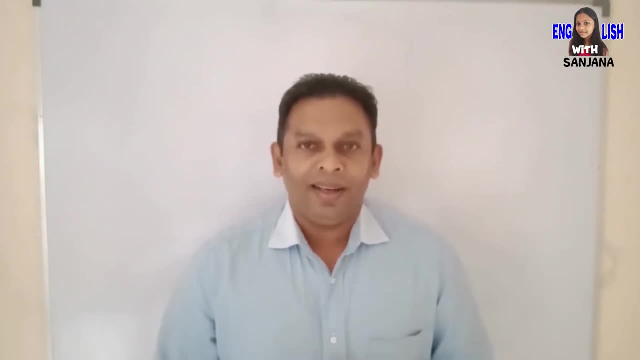 included lots of colorful and relevant pictures and maps for your quick and easy understanding. If you stay tuned until the end of this presentation, I am pretty sure you can have a better understanding on the population distribution in the Asian region. Then join me in this lesson on the. 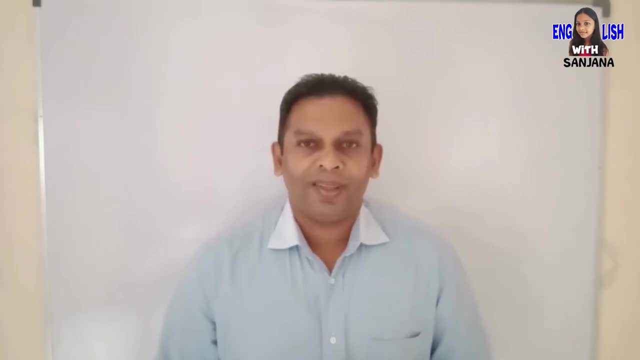 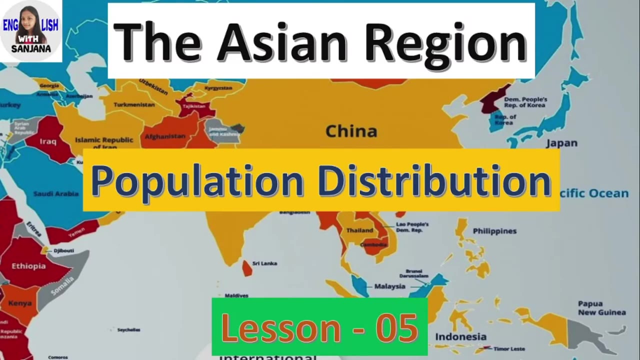 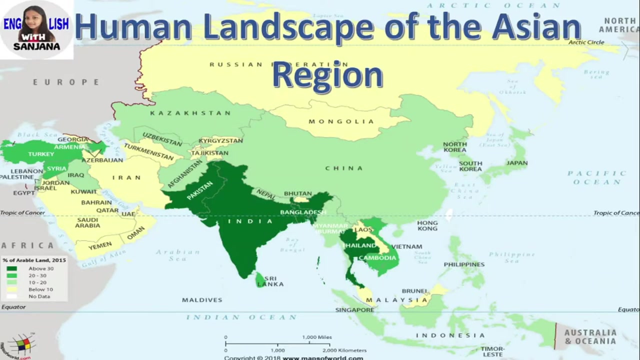 Asian region and its population. If you are ready, let's get started. The Asian Region Population Distribution- Unit 1, Lesson 5. In my previous videos on the Asian region we already discussed much information on the geographical location of Asia, physical landscape of Asia and human landscape of Asia. Under. 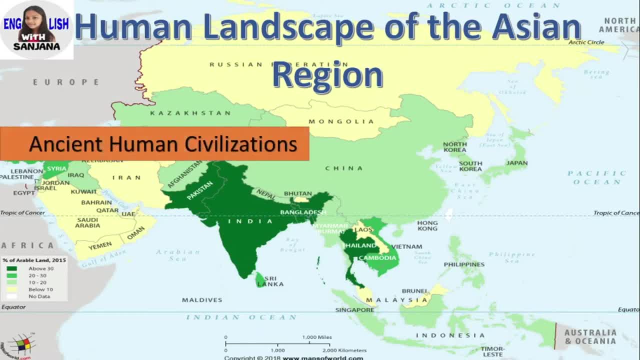 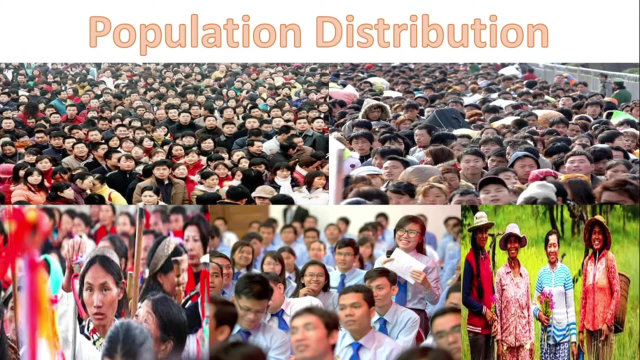 human landscape of Asia. we already learned about ancient human civilizations and types of human races in Asia. In this video, we will have a sharp and quick focus on Population Distribution in Asia. Population distribution is a critical phenomenon which can be used to determine whether any 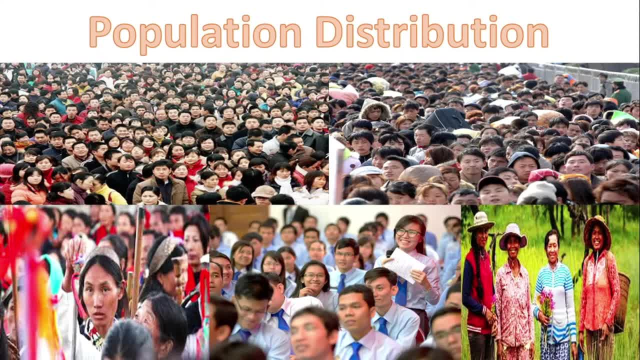 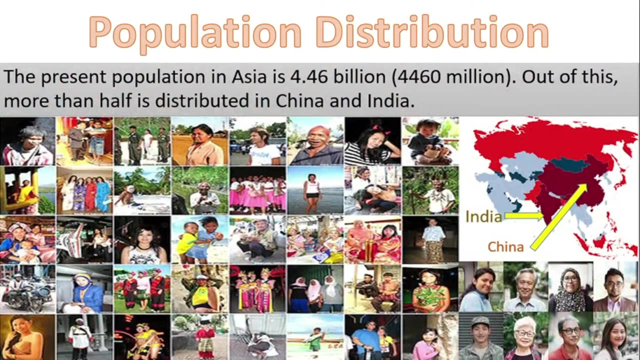 region in the world has reached its own limitations in terms of population and its distribution. Population distribution means how humans have spread geographically on the surface of the Earth. The population in Asia is more than 4.46 billion. Out of this, more than half is distributed. 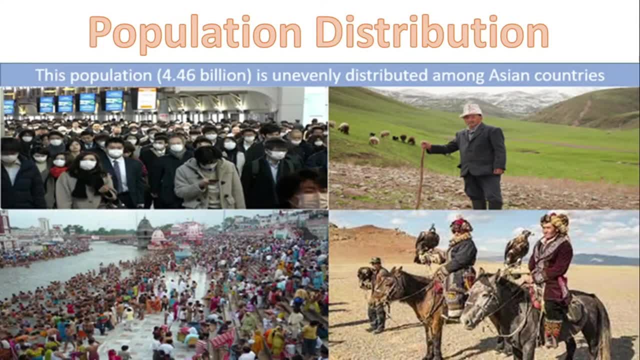 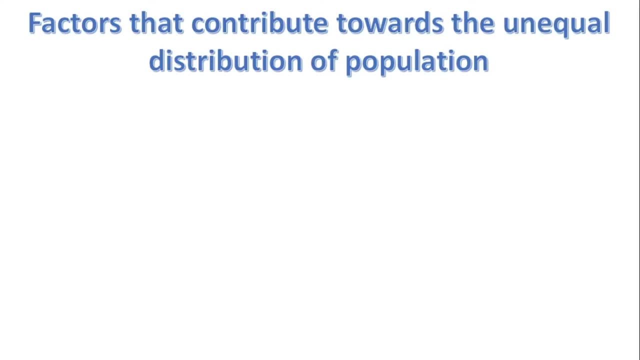 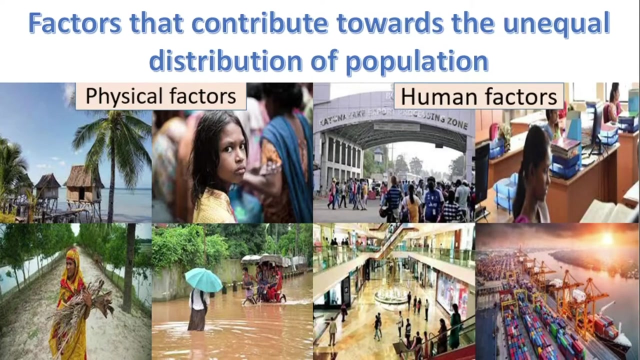 in China and India. This population is unevenly distributed among Asian countries. There are many factors that have contributed for the unequal distribution of population. These factors can be divided into two categories. They are physical factors and human factors. In this presentation on population distribution in Asia, we are not going to pay our attention. 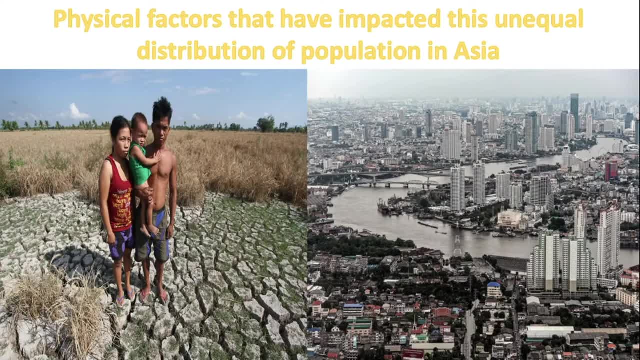 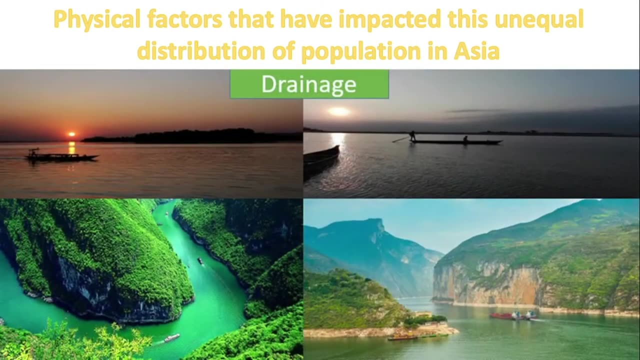 to human factors. We will only be looking at physical factors. What are the physical factors that have impacted this unequal distribution of population in Asia? They are relief features, climate drainage and soil, In addition to these distribution of natural resources and 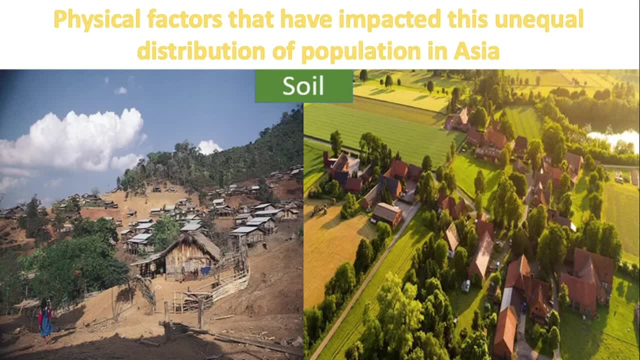 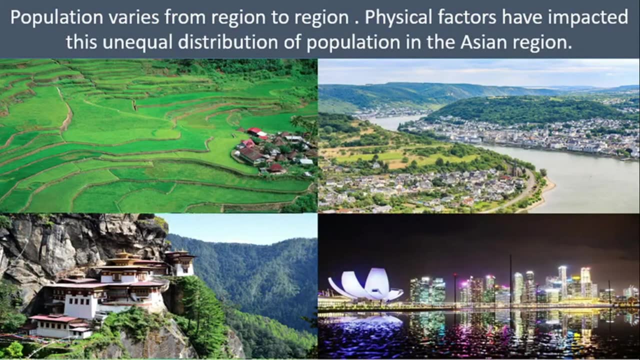 natural resources In addition to these, distribution of natural resources and natural resources. In addition, distribution of natural resources and natural resources and natural resources. We can see that the nature and vegetation are also factors that affect population distribution. So population varies from region to region. Physical factors have mainly impacted this unequal distribution. 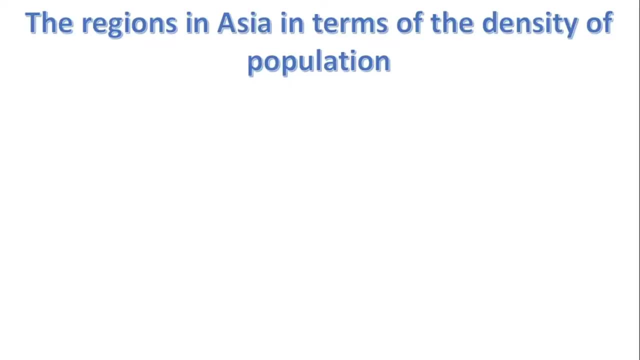 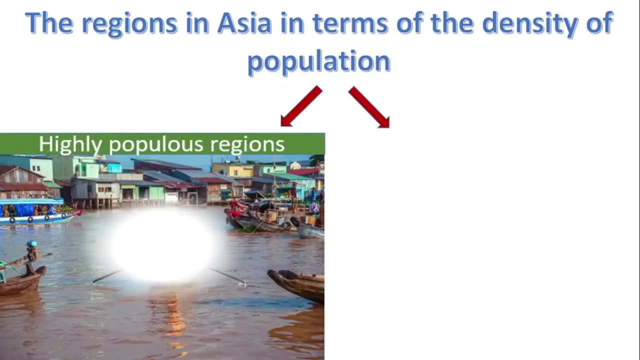 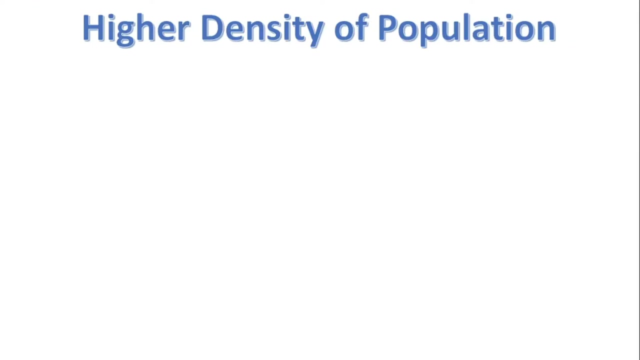 of population in the Asian region. Now let's look at the regions in Asia in terms of the density of population. Some regions are highly populated, whereas some regions are sparsely populated. As you, sparsely populated when considering the population in asia based on the density of population. 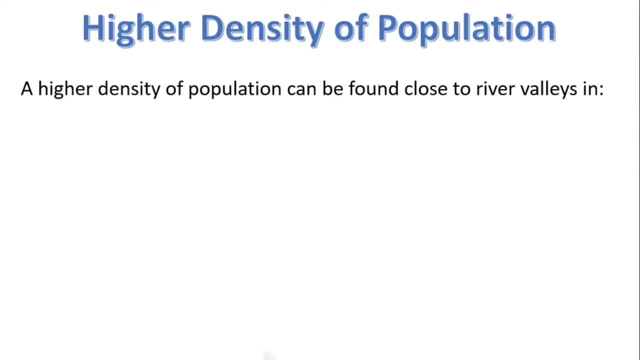 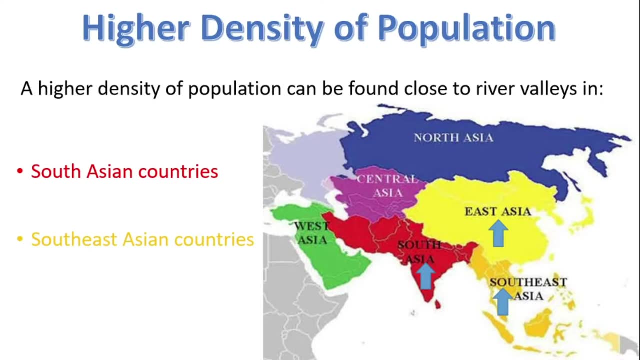 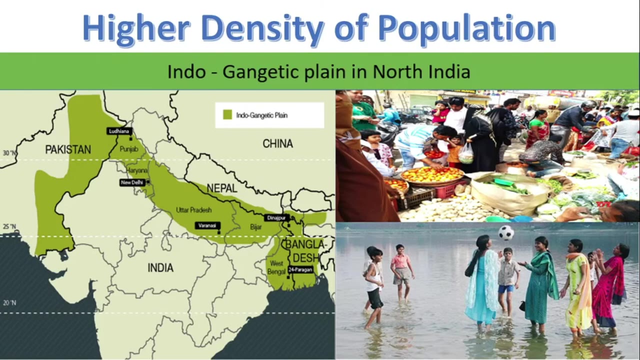 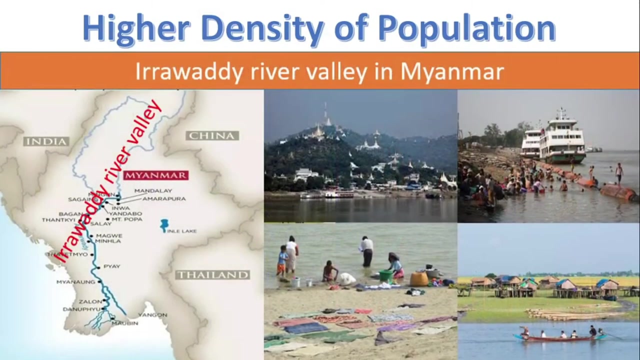 a higher density of population can be found close to river valleys in south asian countries, south east asian countries and east asian countries in. the gangetic plane in north india is an example for a river valley in south asia which holds a higher density of population. irreverent river valley in myanmar is such example for a river valley in southeast asia. 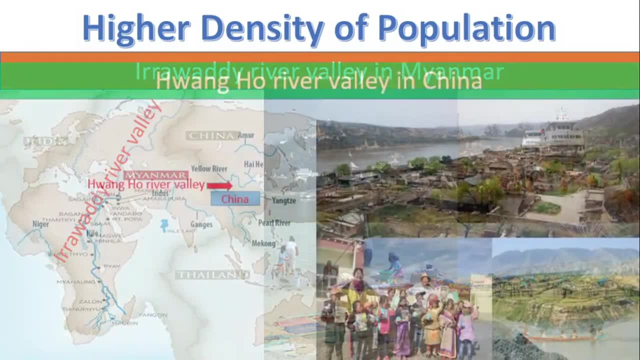 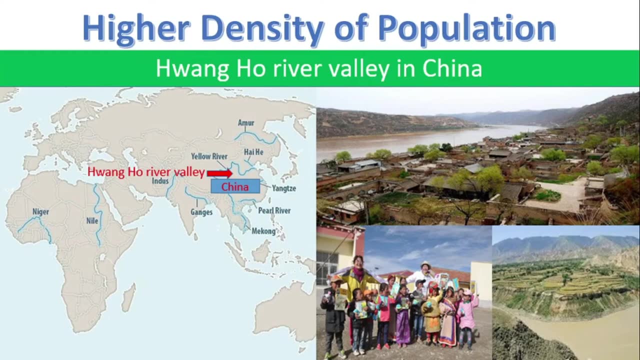 which is home for higher density of population. guangzhou river valley in china is, too, a significant example for a river valley in east asia which shelters a higher density of population. these areas are very special examples for river valleys with a higher density of population in asia, not 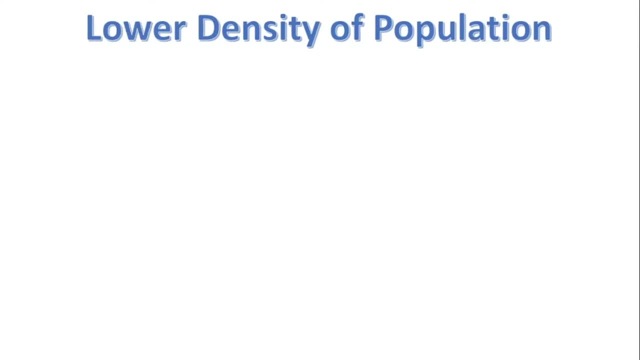 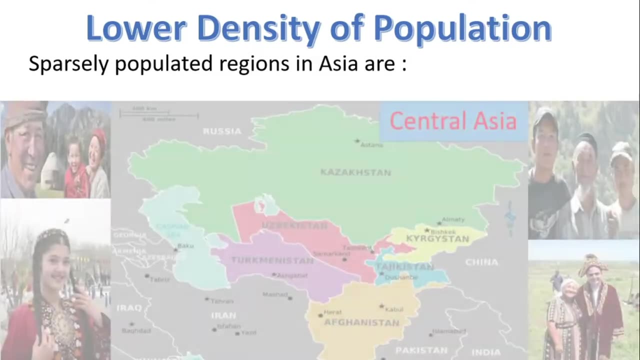 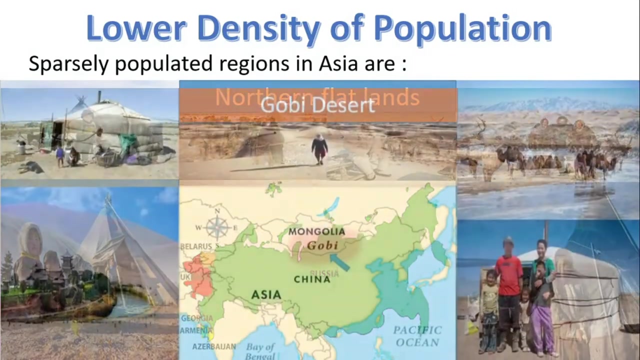 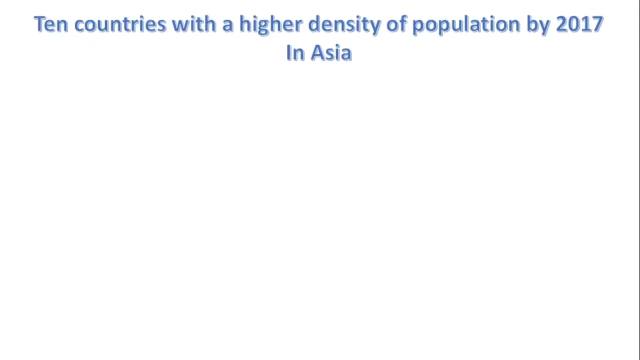 only that, some areas can be cited in asia with a lower density of population. sparsely populated region in asia are: central asia, mongolia, northern flatlands, gobi desert, thar desert. now it's time to remind you of 10 countries with a higher density of population by 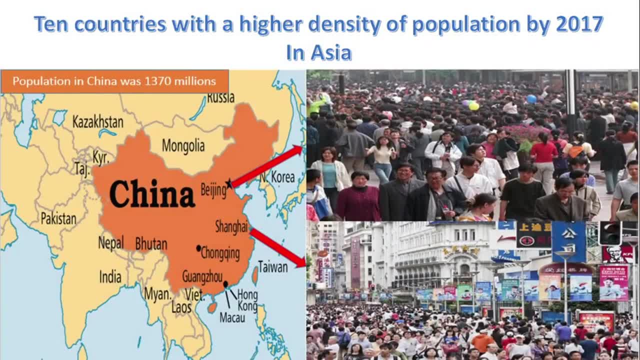 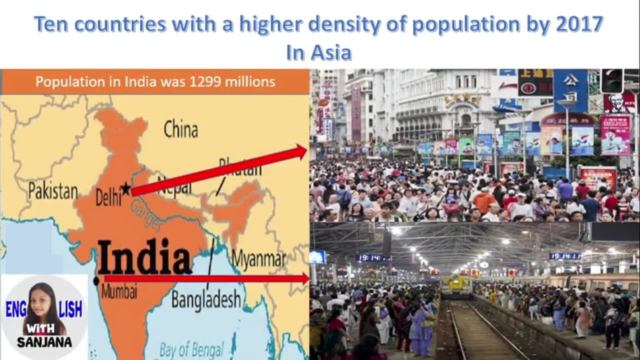 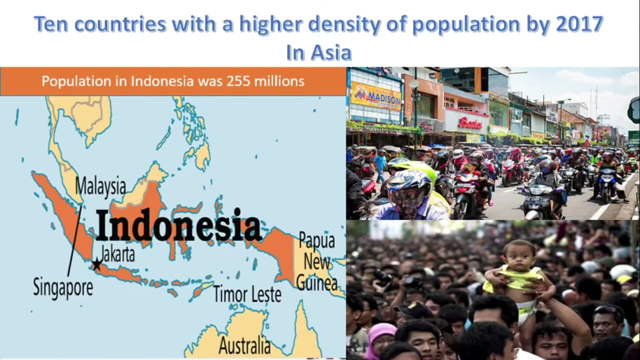 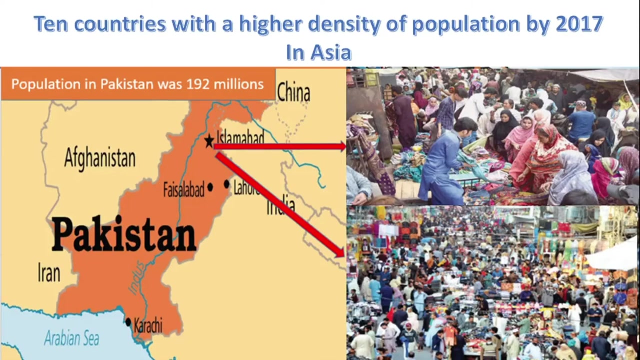 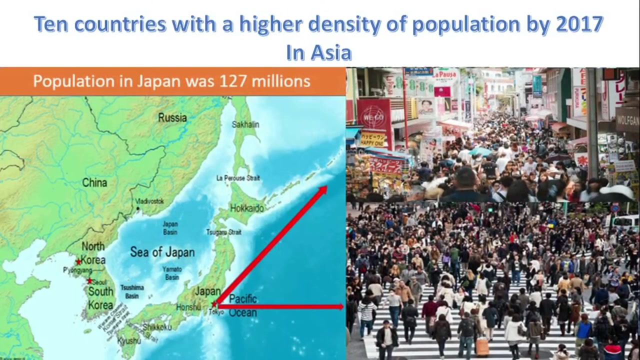 2017 in asia: population in china: it was 1370 millions. population in india: it was 1299 millions. population in indonesia: it was 255 millions. population in pakistan: it was 292 millions. population in bangladesh: it was 159 millions. population in japan: it was 127 millian. 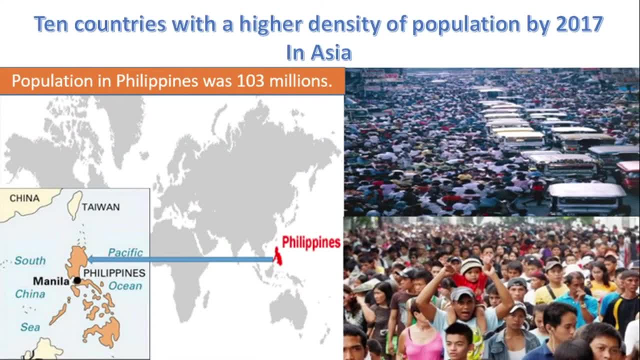 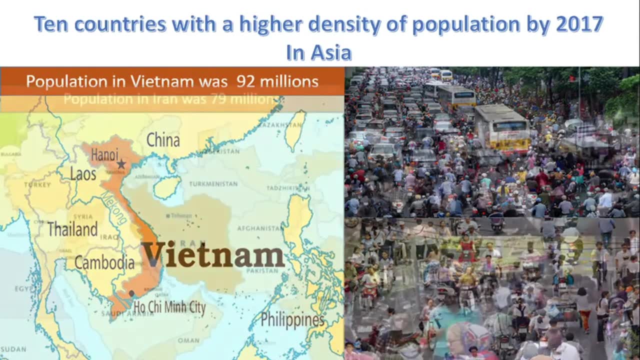 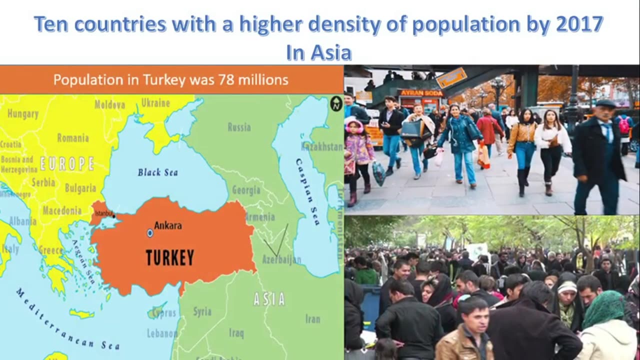 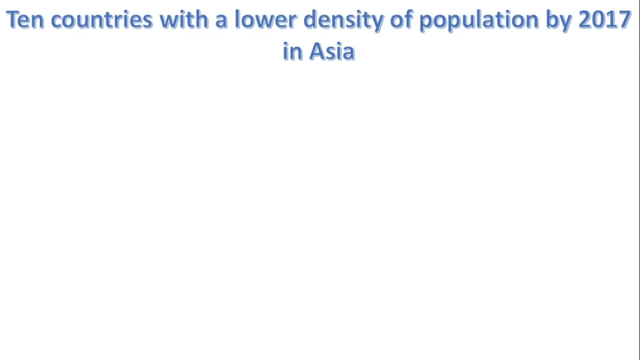 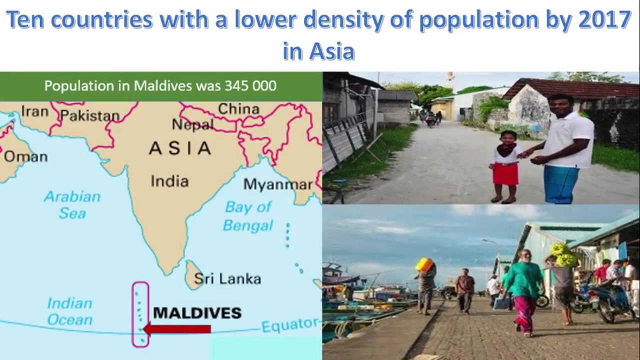 India: it was 207 million. it was 192 million population. inturkey, it was 173 million- 78 millions. now we pay our attention to 10 countries with a lower density of population by 2017. in Asia population in Maldives: it was 345 thousand population. 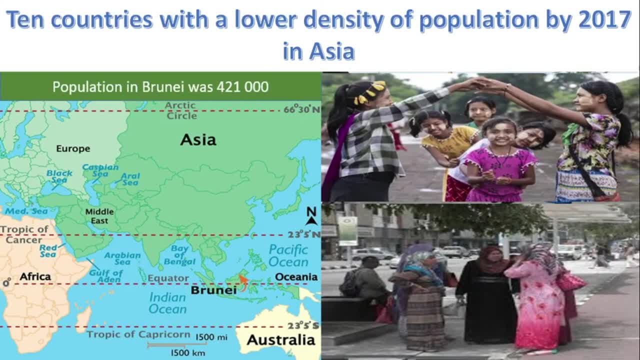 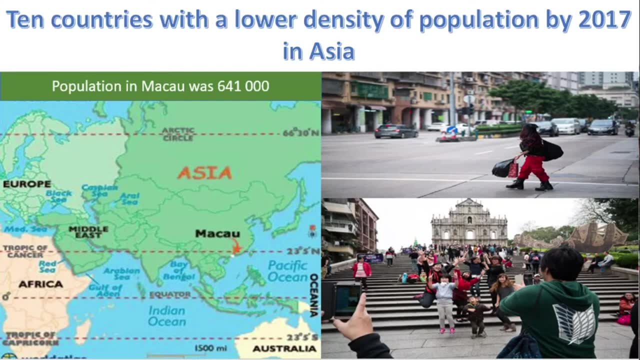 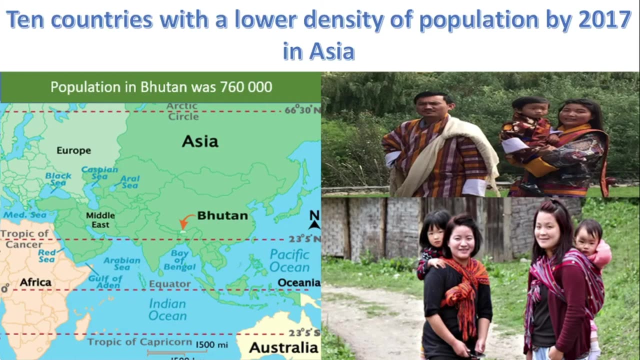 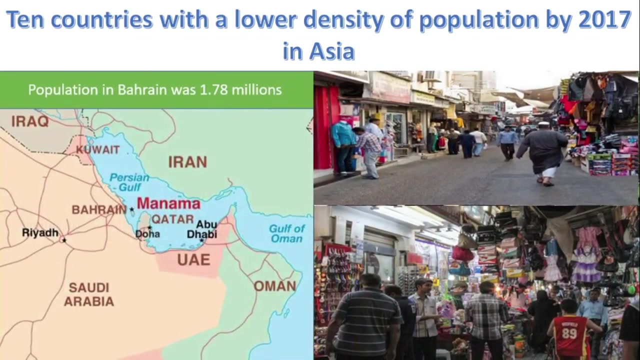 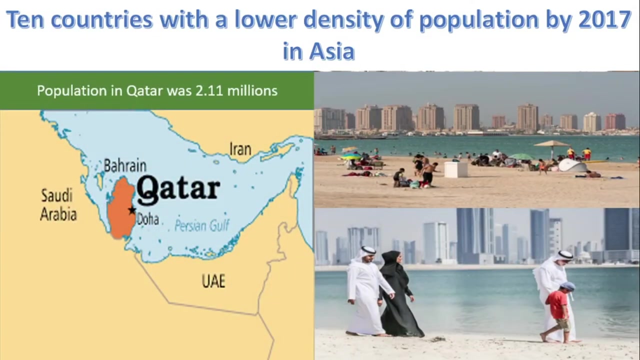 in Brunei: it was 421 thousand. population in Macau: it was 641 thousand. population in Bhutan: it was 760 thousand. population in Timor: 1.24 millions. population in Bahrain: it was 1.78 millions. population in Qatar: it was 2.11. 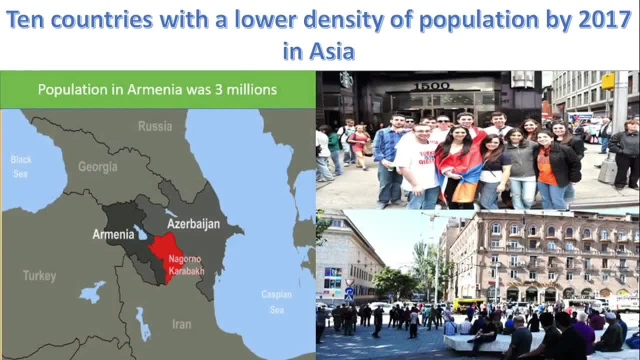 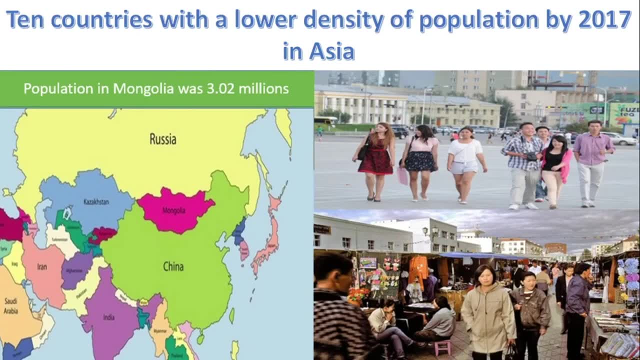 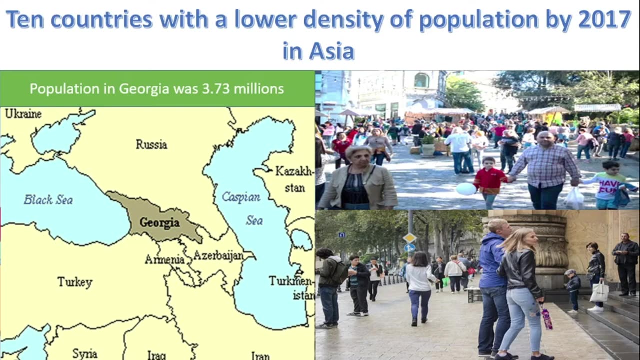 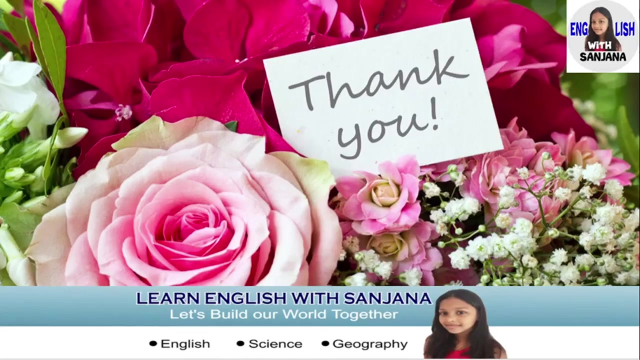 millions. population in Armenia: it was 3 millions. population in Mongolia: it was 3.02 millions. population in Georgia: it was 3.73 millions. this is the end of our presentation on population distribution. with this presentation we conclude human landscape in the Asian region. thank you very much for watching.